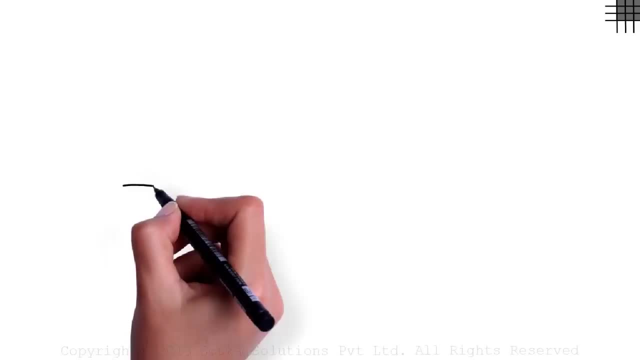 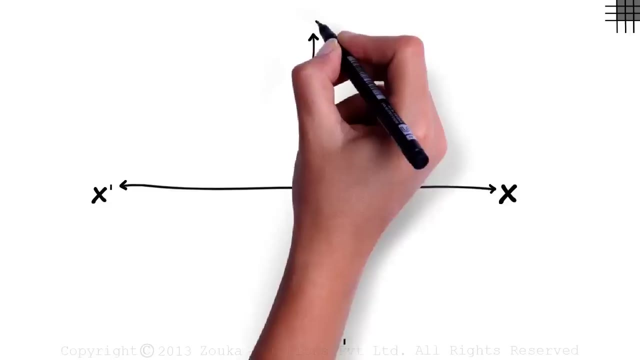 So we draw the x-axis and name it x dash x. We draw the y-axis and name it y dash y. How do we number the axis? Until now, we have only seen cases where we have numbered this side of the x-axis and this side of the y-axis. 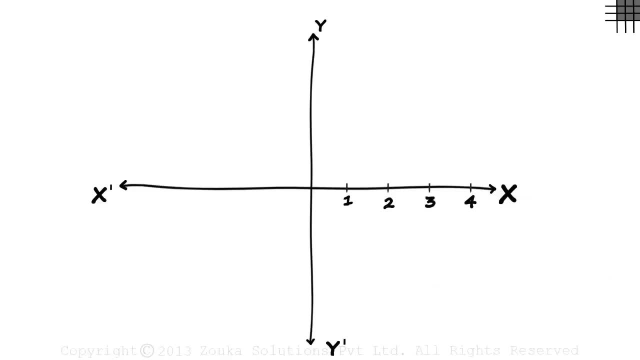 One, two, three, four and so on on the x-axis, And one, two, three, four and so on on the y-axis, The reference point or the origin is zero. On the left hand side of the horizontal axis, just like the number line, we mark negative natural numbers. 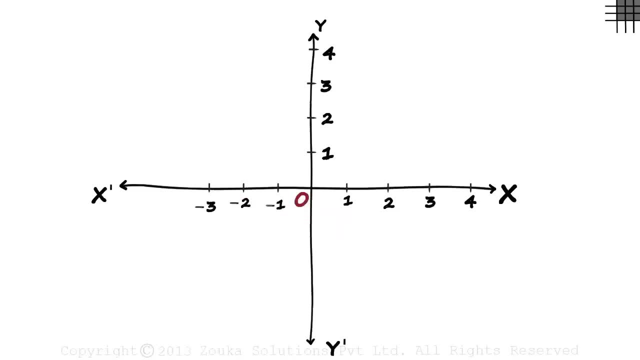 minus one, minus two, minus three, minus four, and so on. Similarly, on this side of the y-axis we mark minus one minus two, minus three, minus four, and so on. Remember, all these are marked in equal intervals. 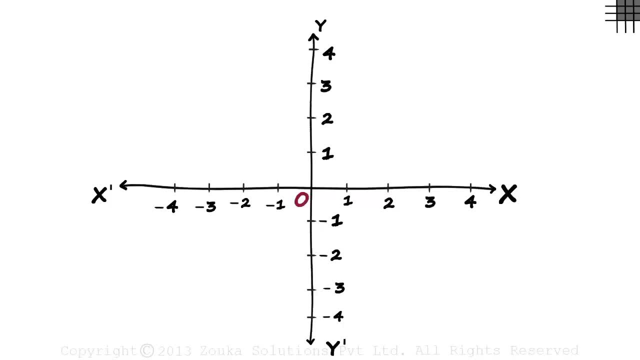 Now let's take a random point somewhere on the plane and try to give it an identity. Say we have a point P here. It is three units away from the origin on the horizontal axis and two units away on the vertical axis. How do we denote the point then? 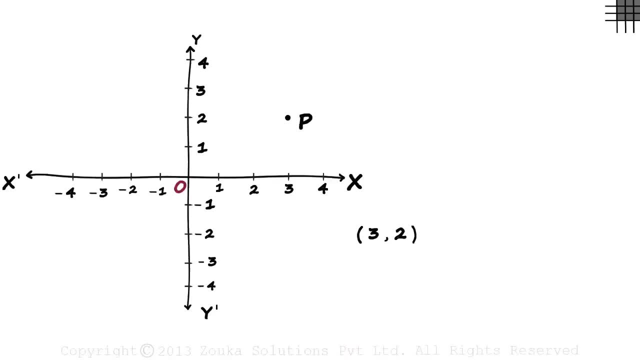 We write it as inside round brackets. That's the identity of point P, But in mathematics we do not refer to it as an identity. We call these the coordinates of point P. Three is the x-coordinate and two is the y-coordinate. 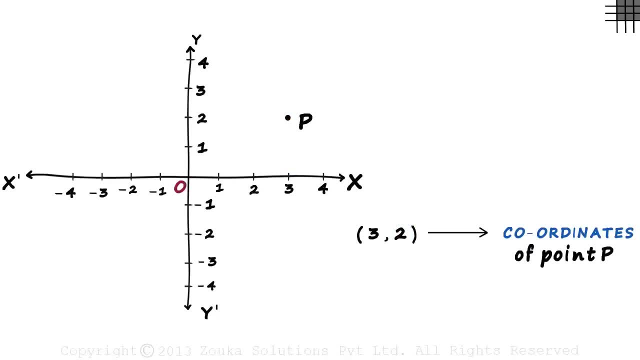 Here's something you really need to know. This is not the same as will be this point here, Two units away on the x-axis and three units away on the y-axis. The order matters, Hence they are called an ordered pair. The value on the x-axis is always written first.